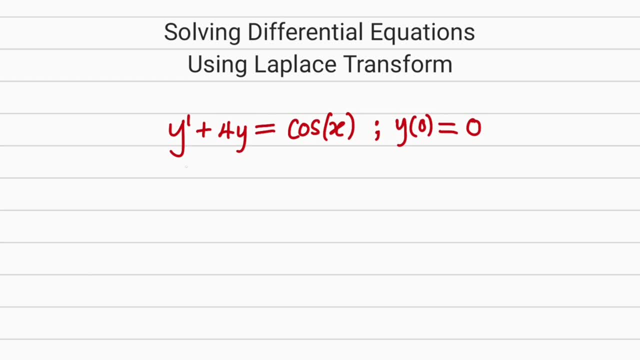 the Laplace transform of each of these times, We have the Laplace transform of y prime, plus the Laplace transform of 4y equals the Laplace transform of cosine x. The Laplace transform of y prime is the same thing as s multiplied by the Laplace transform of y. 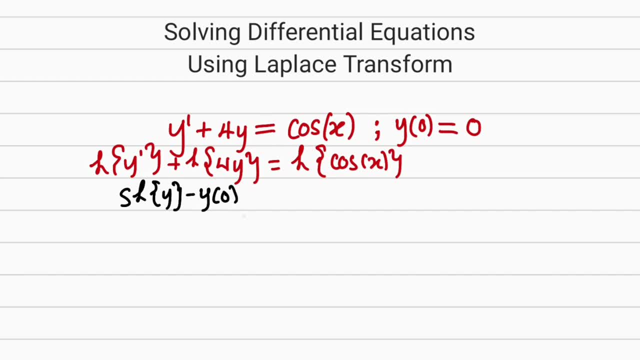 the minus y of 0. Plus, then we take the Laplace transform of the second time, Which is 4y. We can bring out 4 and take the Laplace transform of y. All right to the right hand side we have cosine x. But remember, if you have Laplace transform of, 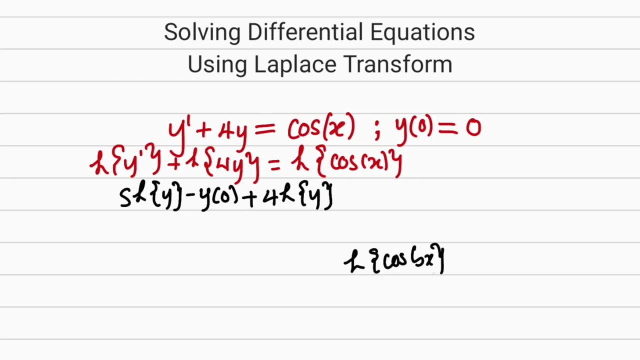 cosine bx. it is the same thing as s divided by s squared plus b squared b is the coefficient of x. Therefore, this is the Laplace transform of y. We can bring out 4 and take the Laplace transform of y. 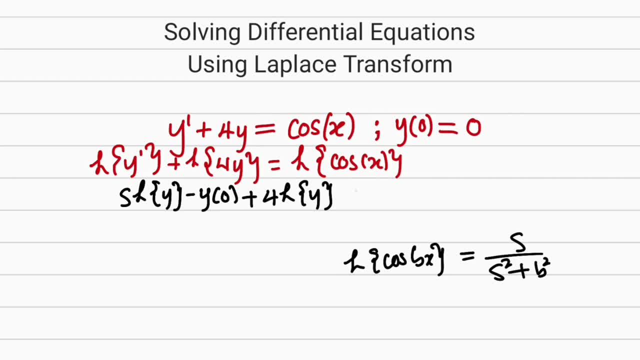 This time around we have 1 as our coefficient. Therefore this becomes s divided by s squared plus 1.. Because 1 squared is the same thing as 1.. Then, for the initial condition, you can see that y of 0 is equal to 0.. 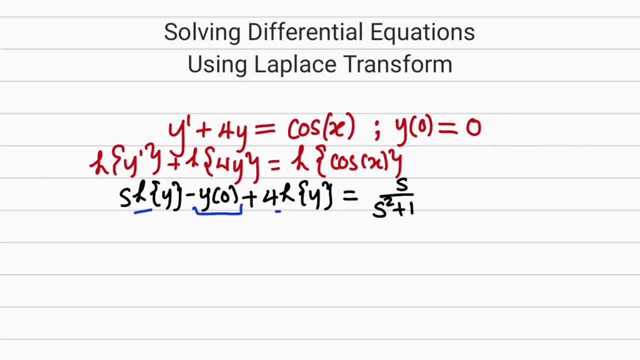 Therefore, this term here becomes 0.. All we have is this and this, Which we can factor out, the Laplace transform of y, So we have s plus 4.. Multiply by the Laplace transform of y And, to the right hand side, we have s divided by s squared plus 1.. 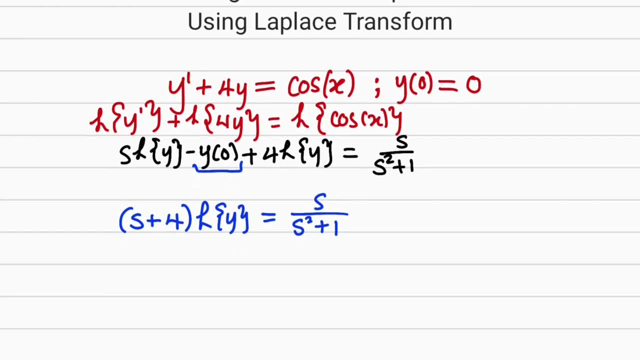 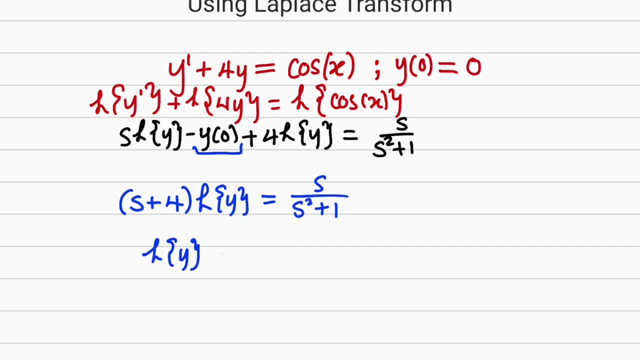 Now we can divide both sides by s plus 4.. Just to have the Laplace transform of y to the left, The Laplace transform of y is equal to s divided by s plus 4.. Multiply by s squared plus 1.. Now we have a compound fraction that we need to dissolve into partial fractions. 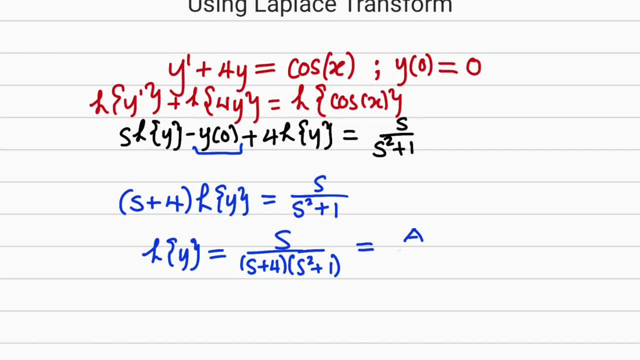 And this is equal to a divided by the first factor, s plus 4.. Because it is a linear factor Plus bs, plus c, divided by s squared plus 1. This quadratic factor is irreducible. Therefore we have to have a linear polynomial to the top. 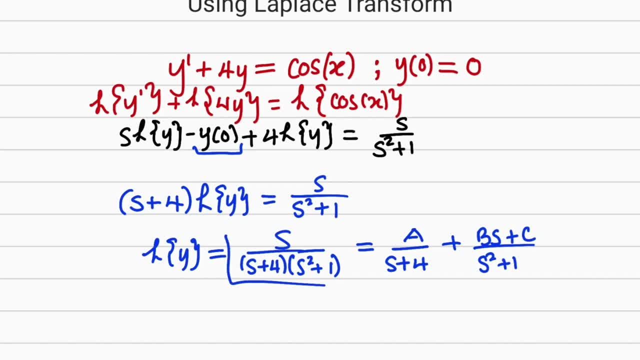 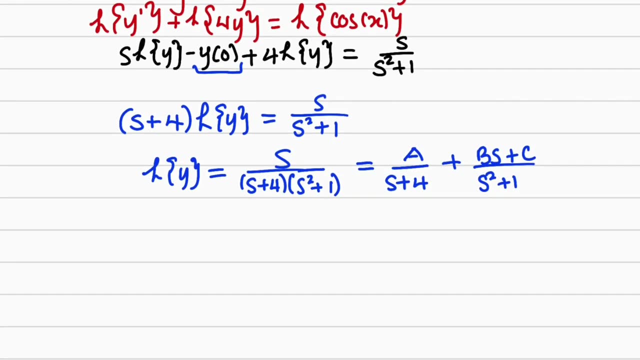 All right, This is what we have to solve first, before we take the inverse Laplace transform of it. Let us first of all multiply each term by these two factors in order to clear the fractions To the left hand side. we have just s if multiplied by the two factors. 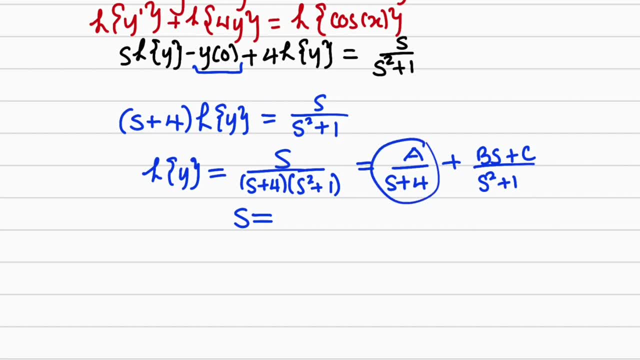 And to the right hand side. if you multiply this by the two factors s plus 4 will cancel s plus 4.. All we have is a multiplied by s squared plus 1.. Plus Take this: multiplied by these two factors: s squared plus 1 will cancel s squared plus 1.. 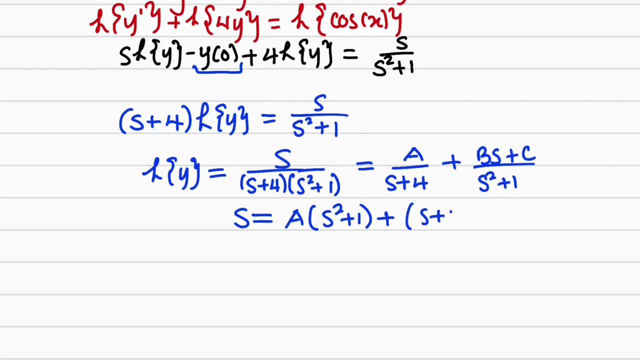 All we have left is s plus 4.. Then multiplied by our numerator here, Which is bs plus c. Now let us expand this parenthesis s to the left, and we have a s squared plus a. if a is distributed Plus s multiplied by bs, we have bs squared. 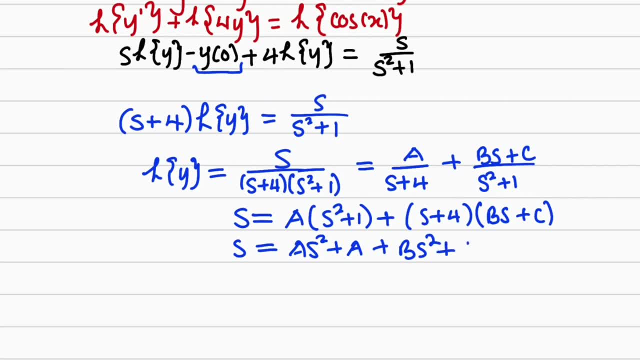 s multiplied by c, we have cs. Then we take the second term, 4 multiplied by bs, we have 4bs. And lastly, 4 multiplied by c is 4c. To the left we have s And to the right we can bring those with s squared together. 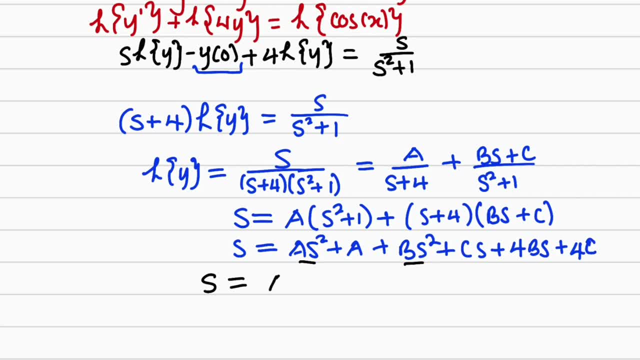 We have one here and we have the other one here. Therefore, we have a plus b Multiplied by s squared. We just factor out s squared Plus, Then we take those with s. We have one here and we have the other one here. 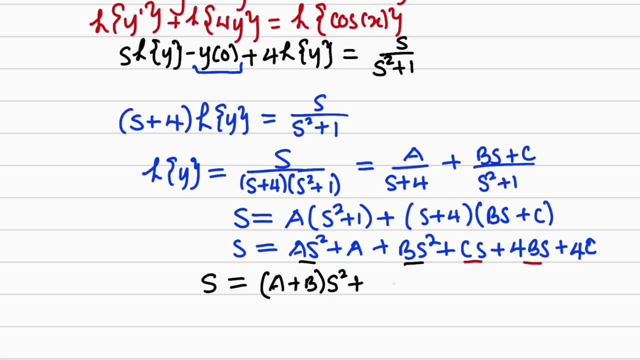 So this is 4b plus c. I want to write it in order: 4b plus c multiplied by s. Then the last one: we have the two constants a and 4c. a plus 4c. Alright, Now let us solve this equation by relating the coefficients. 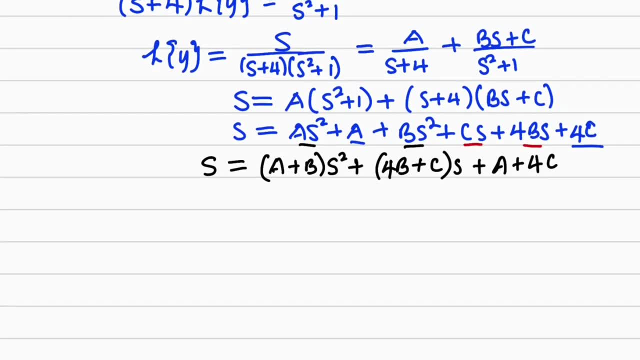 The coefficient of s squared to the right is a plus b, And the coefficient of s squared to the left is 0, because we do not have any s squared here. Then we move on. The coefficient of s to the right Is 4b plus c. 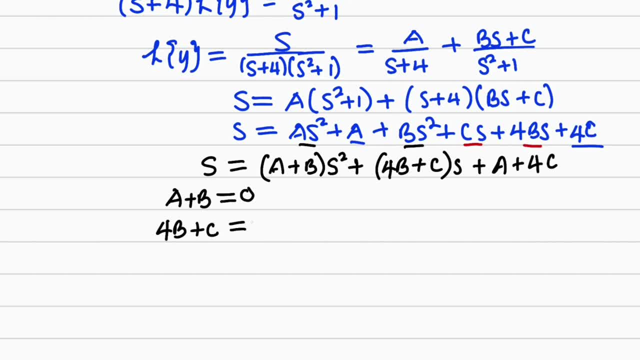 And that of the left hand side is 1.. Then the constants: We have a plus 4c equals 0, because we do not have any constant to the left. Alright, Here are our three equations. Alright, From equation 1.. 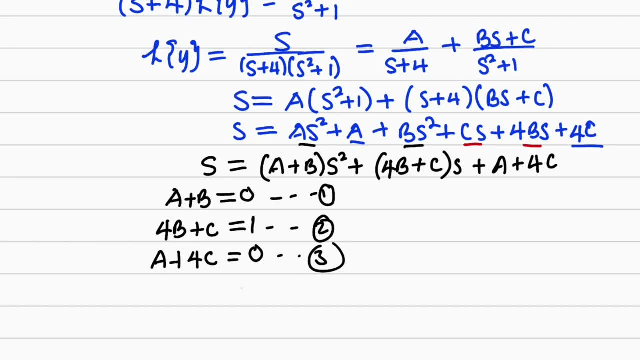 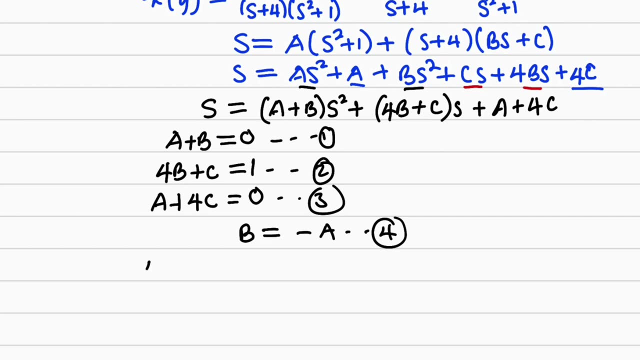 We can make b the subject. Therefore b is the same thing as negative a. So we can substitute this negative a into the second equation. From the second equation we have 4 multiplied by b, But b is negative a. So we have negative for a plus c. 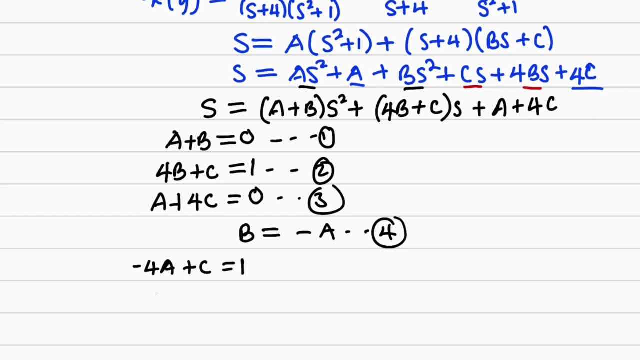 And this is equal to 1. Then we can bring equation 3. We can even multiply that with 4.. So we have: 4 multiplied by a is 4a, Then 4 multiplied by 4c is 16c. 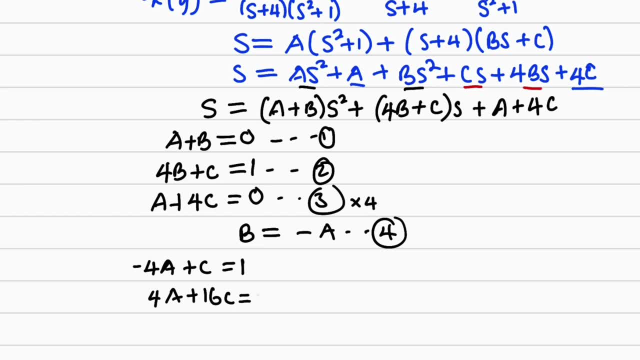 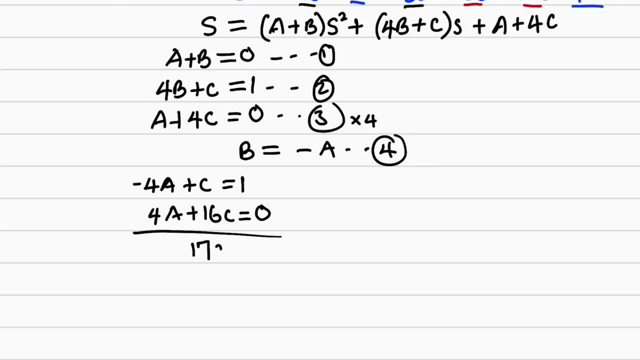 And to the right hand side, we have 4 multiplied by 0, equal to 0.. Let us add these two equations together, We have 17c Equal to 1.. Because negative 4a plus 4a is 0.. 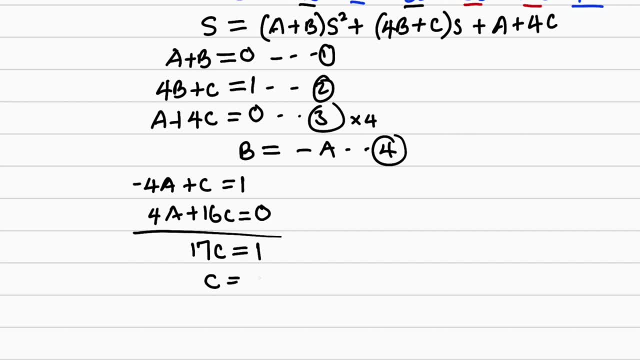 Divide both sides by 17.. We have c equal to 1 divided by 17.. Alright, Let us plug it back into one of these equations. Let us plug it back here: a plus 4c equal to 0.. a plus 4 multiplied by 1, divided by 17.. 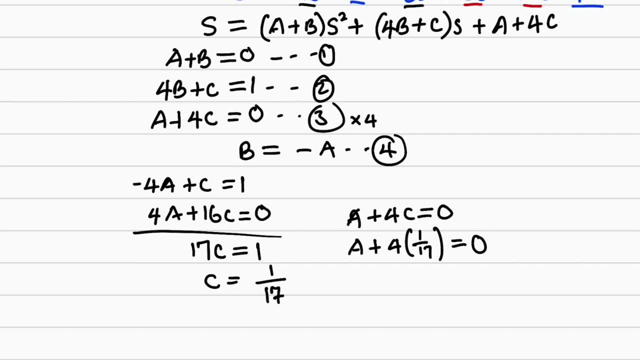 This is equal to 0.. Let us multiply both sides by 17 to clear the fraction. We have 17a plus 4, equal to 0.. We can take 4 to the right, So we have 17a equals negative 4.. 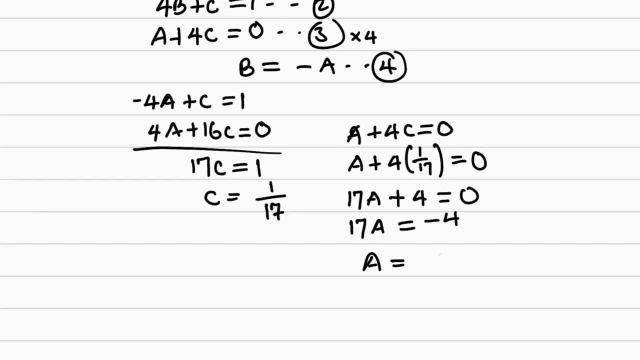 Therefore, a is equal to negative 4 divided by 17.. All we have to find next is b, But b is negative a. We can just multiply a by negative to get the value of b. Therefore, b will be equal to positive 4 divided by 17.. 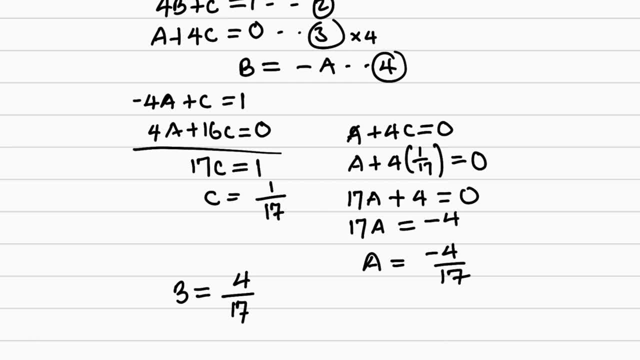 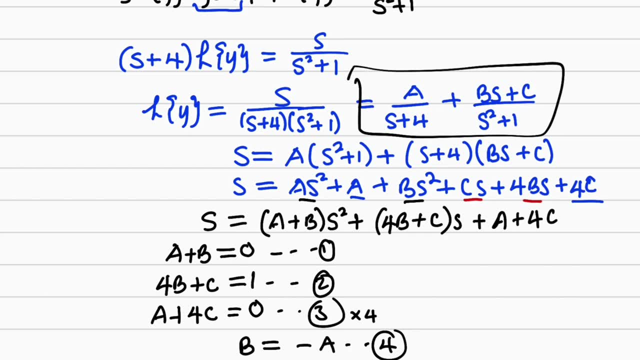 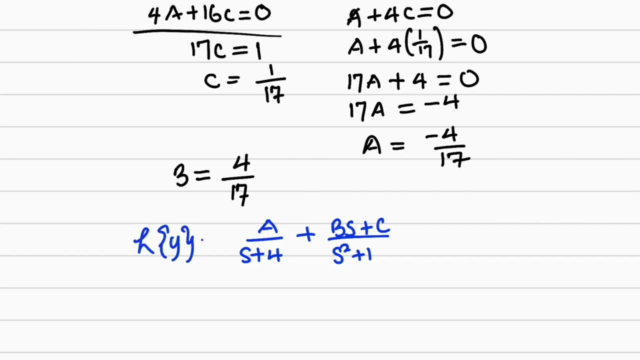 Okay, Now we have a, b and c. We can plug them back into this equation right here. Okay, Let me copy that. Therefore, the Laplace transform of y is equal to this, which we can substitute: a is negative 4 over 17.. 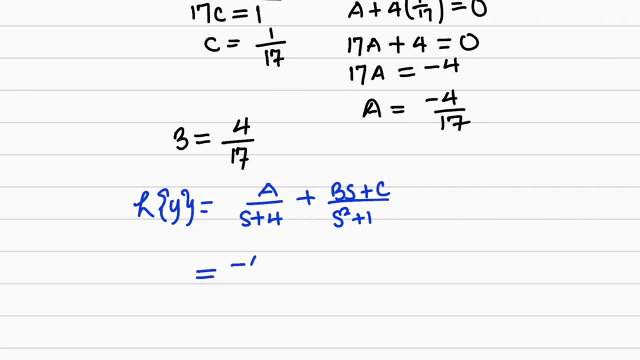 So we have negative 4 divided by 17.. Multiply by 1 divided by s plus 4.. Then we move on. We can even split this. We have: plus b is 4 divided by 17.. So we can write it as 4 divided by 17.. 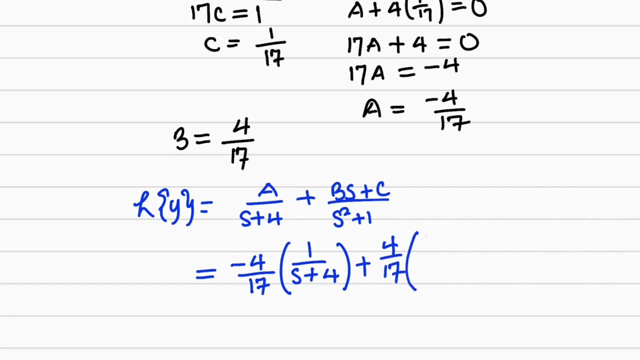 Then multiply by s divided by s squared plus 4.. Then c is 1 divided by 17.. So we can write 1 divided by 17.. Then multiply by 1 divided by s squared plus 1.. I just split this fraction as bs divided by s squared plus 1.. 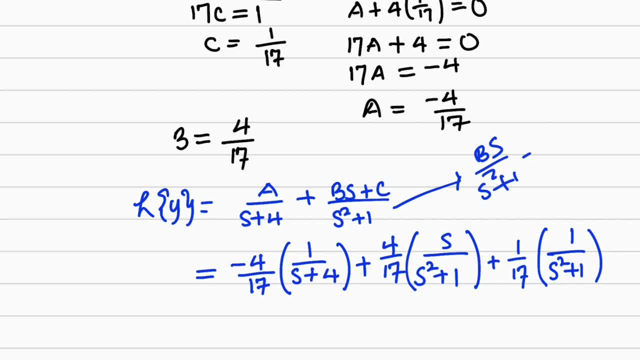 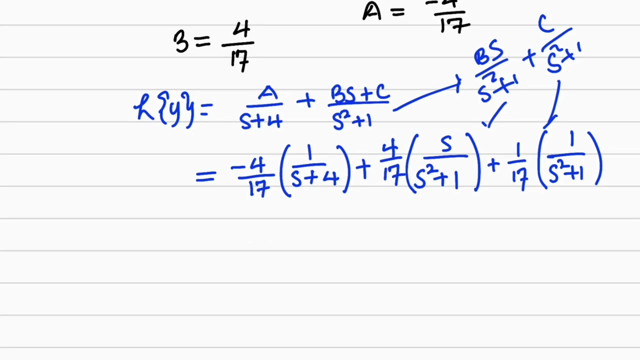 Plus c, divided by s squared plus 1.. That's what I have substituted here. Okay, Now let us continue. Now, all we have to do is to take the inverse Laplace of each of these three terms to get the value of y. 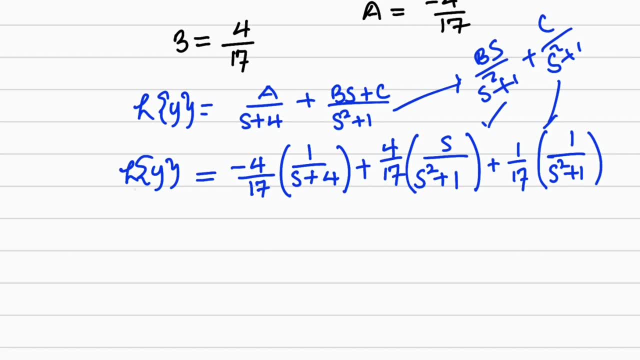 Remember, this is the Laplace transform of y. If you take the inverse Laplace of this, you're going to get y alone. So we have y here, which is a function of x, And this is equal to: We have negative 4 divided by 17.. 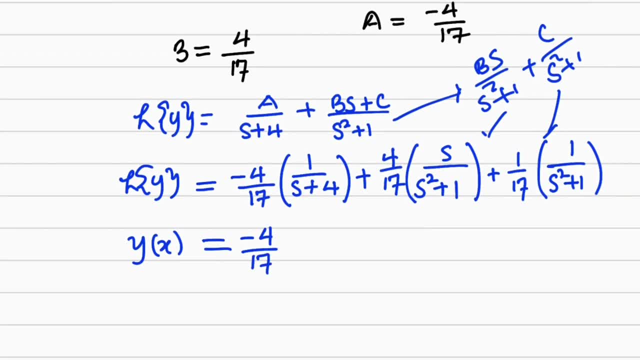 Now, what is the inverse Laplace of this? What I want you to remember is that the Laplace transform of e to the ax is the same thing as 1 divided by s minus 2.. 1 divided by s minus a And a is the coefficient of x. 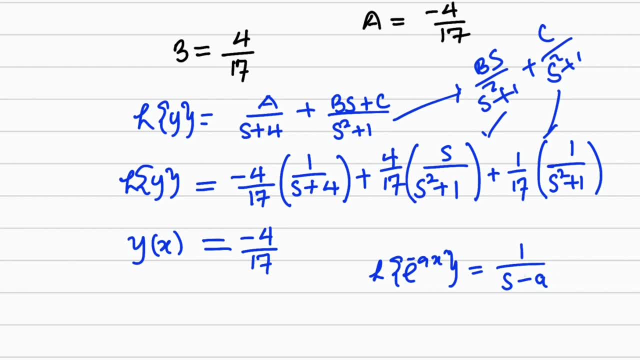 Therefore, if we multiply this a by negative, this will turn to positive, which corresponds to what we are having here. So now the inverse Laplace of 1 divided by s plus 4 will become e to the negative 4x, where a is equal to 4 here. 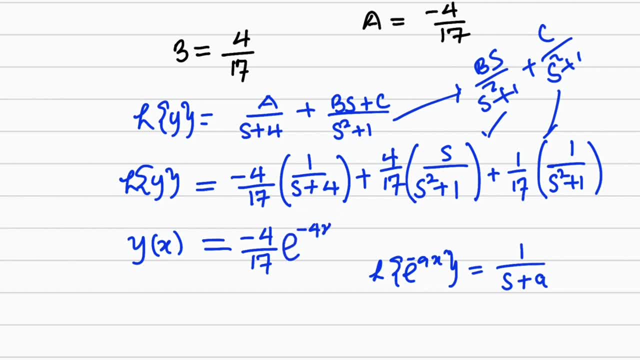 Okay, Negative 4x. Then we move to the second one Plus 4 divided by 17.. All right, The inverse Laplace of this. Remember that again. If you have Laplace transform of cosine bx, This is equal to s divided by.